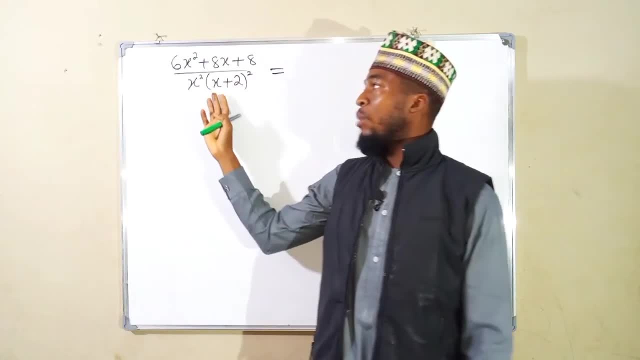 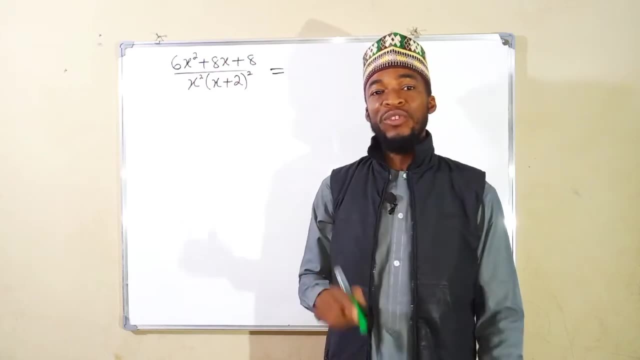 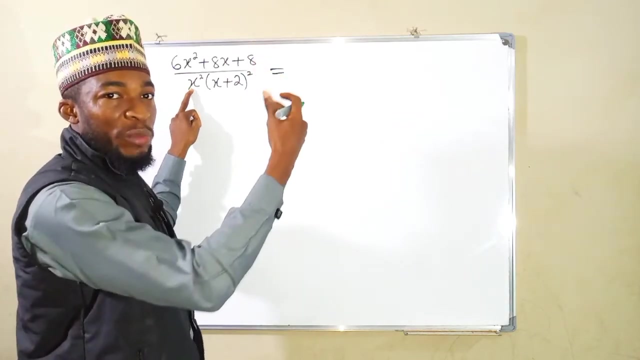 hit the like button. So if you consider this compound fraction it comprises the quadratic and repeated linear factors. So let's see how we are going to transform them. The first one is quadratic factor and therefore each numerator is going to be a polynomial of one degree less than this quadratic factor which is going to 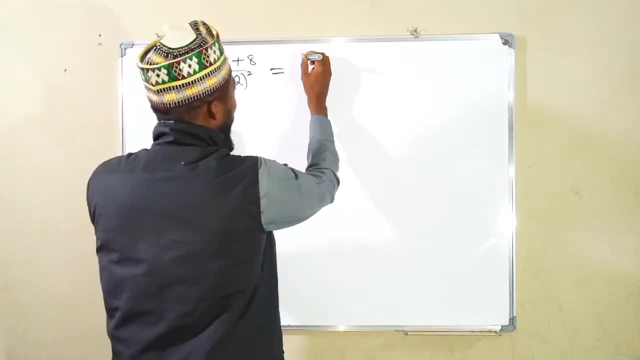 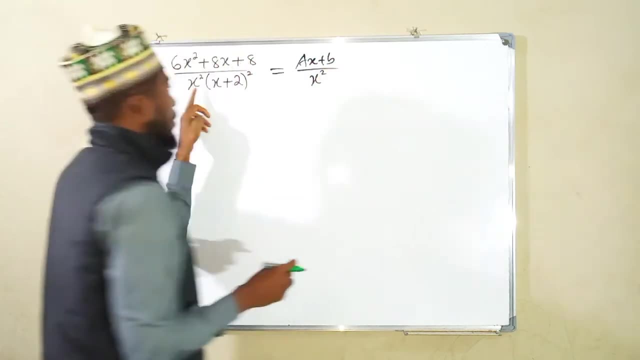 be a linear polynomial, given as ax plus b divided by x squared. Then moving to the next one is repeated factor. In our previous lesson I've shown you how to 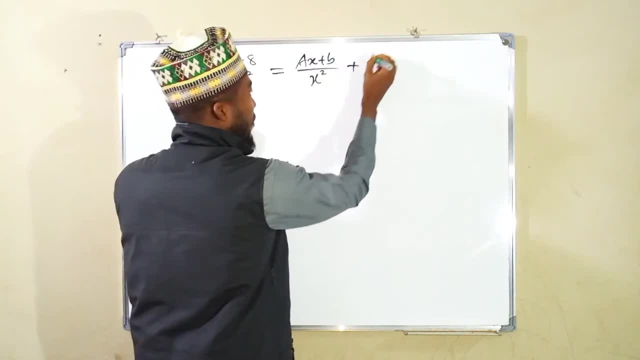 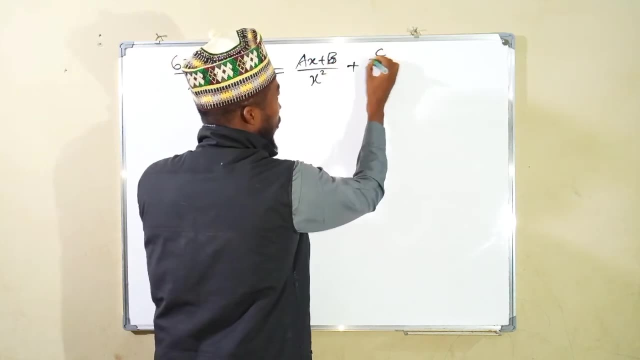 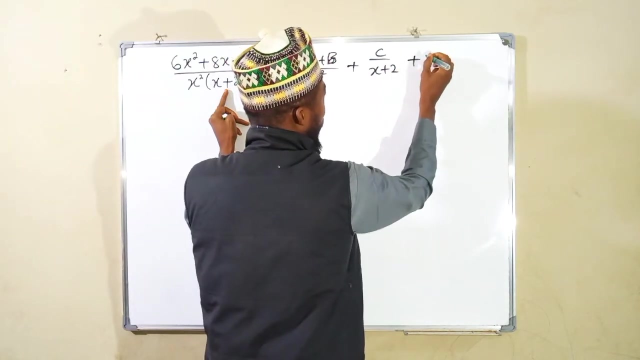 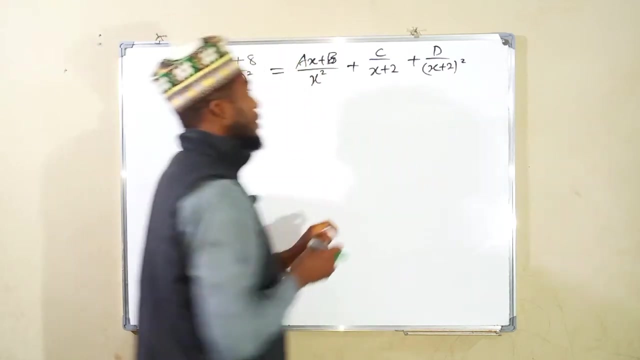 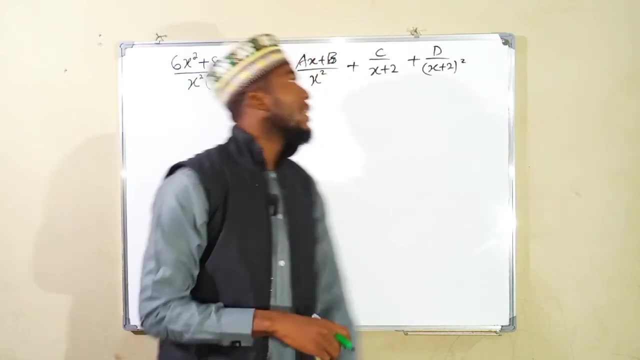 break it down. We first of all take the take a constant to the top. We have used b. Let me even capitalize it. So we are going to say c over x plus 2 to the first power. Then we take another constant, say d over x plus 2 to the second power. If the power is 3, we are going to obtain another constant divided by that linear factor to the last power. So what we are going to do, we are 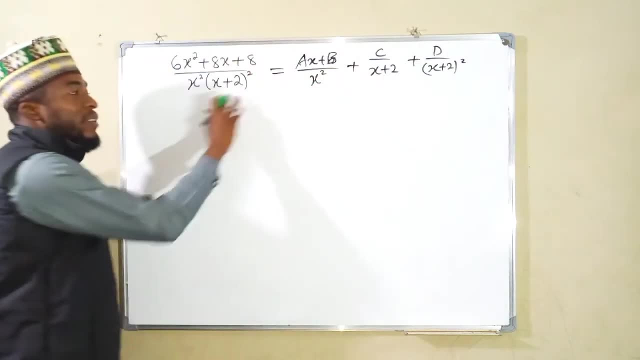 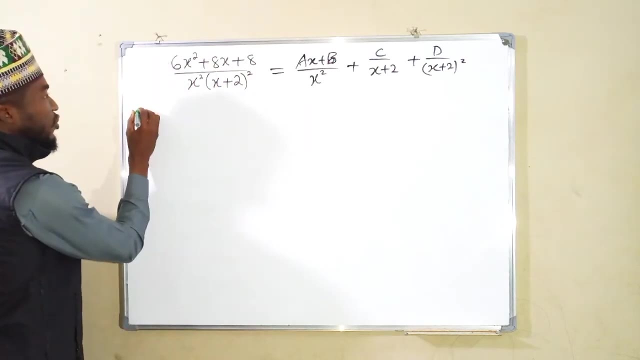 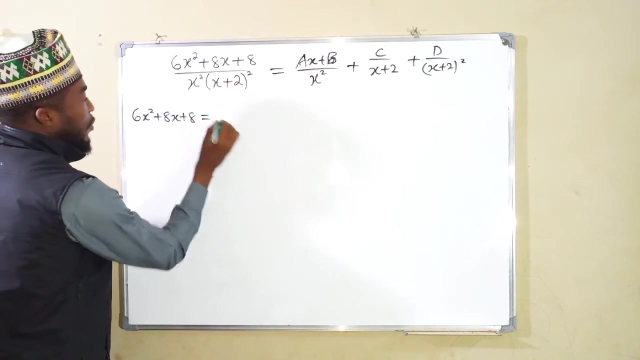 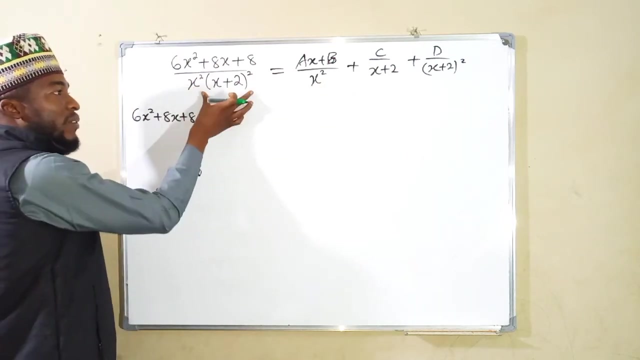 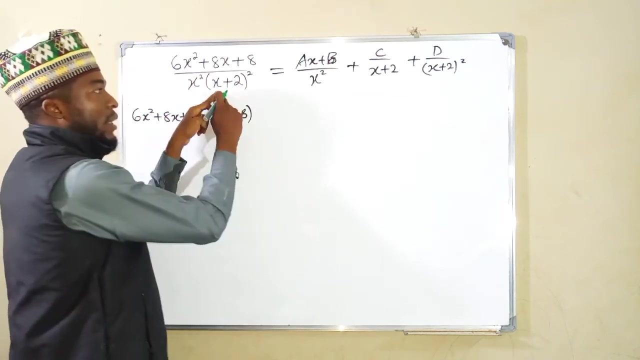 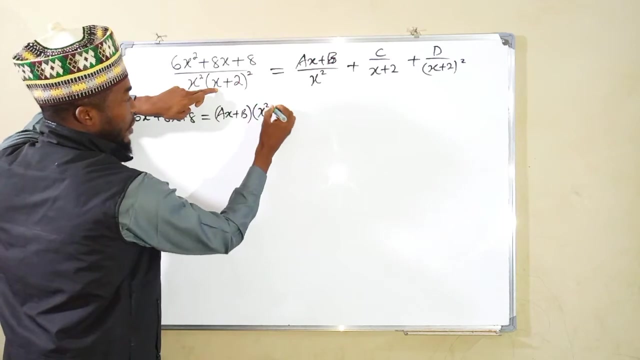 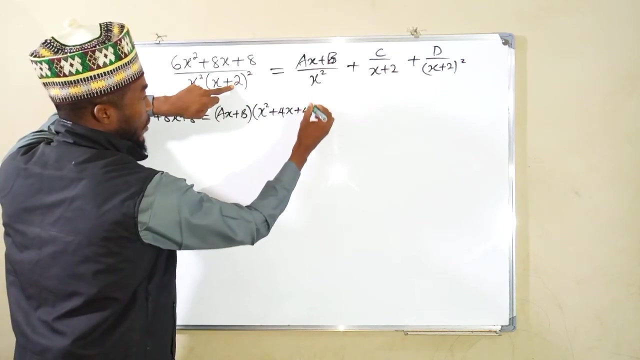 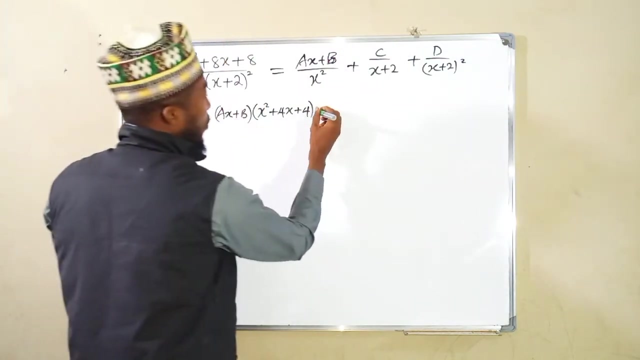 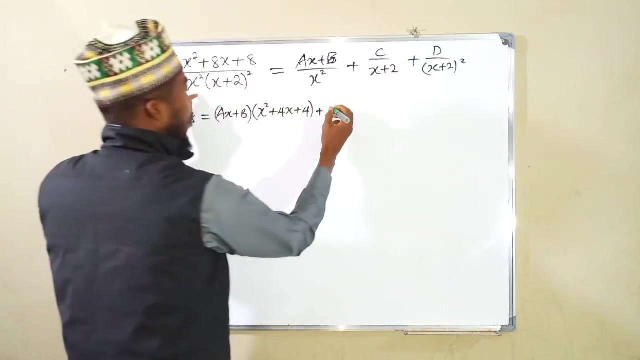 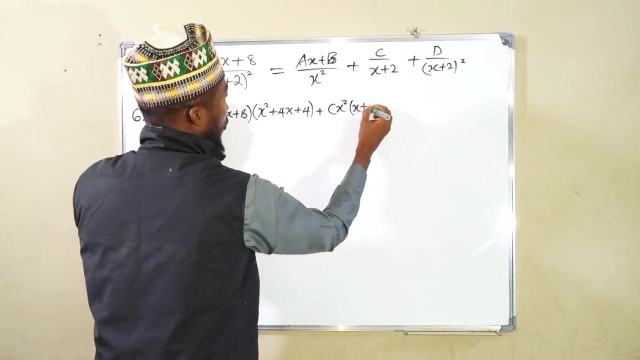 going to multiply each of these fractions by these two factors. Multiplying the left hand side, we are only going to be left with numerator, which is going to be 6x squared plus 8x plus 8. This is equal to, we start with this one, multiplying this by these two factors, this x squared will cancel this. Leaving only this. So we say a x plus b multiplied by x plus 2 to the power of 2. But we can equally expand it from here. First time squared is x squared. 2 times this times this is going to be 4x. Then this squared is 4. Then we will move to the next one. This multiplied by these factors. This is to the power of 1. It will cancel one of it, leaving x plus 2 times x. So we have c times x squared. Then multiply by one of the factors, x plus 2. Plus the last one. 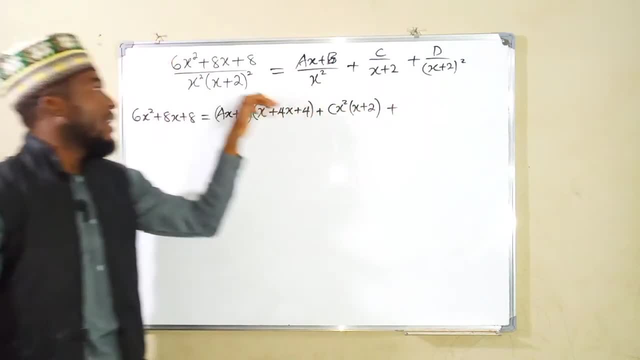 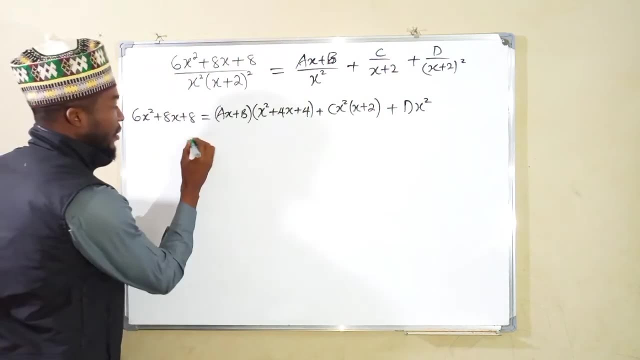 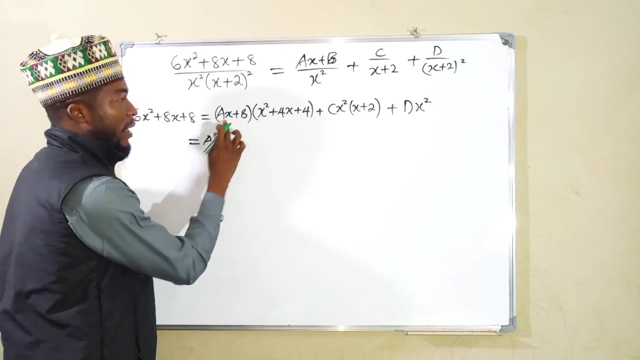 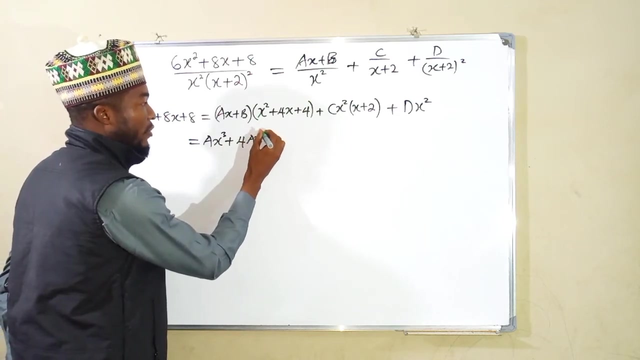 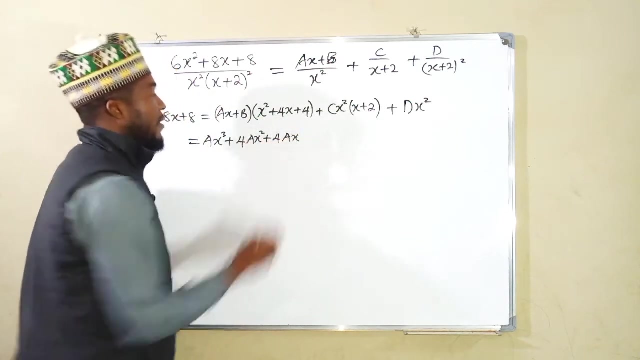 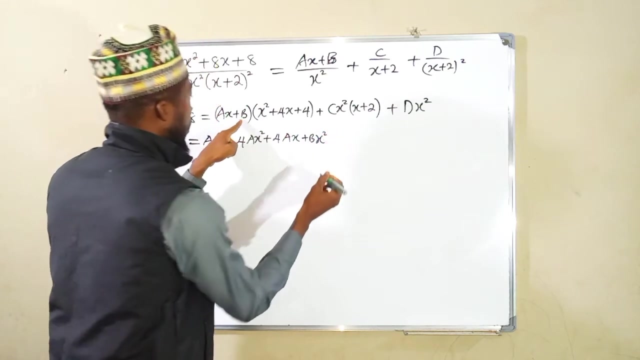 If you multiply the last fraction, this will entirely cancel this, leaving only x squared. Multiply by d, so we have dx squared. Ax times x squared. This is going to be ax squared. This is going to be ax to the third power. Ax times 4x is going to be 4ax to the third power, to the second power, I'm sorry. Ax times 4 is going to be 4ax. Then the second term, d times x squared, we have bx squared. Then b times 4x is going to be 4bx. 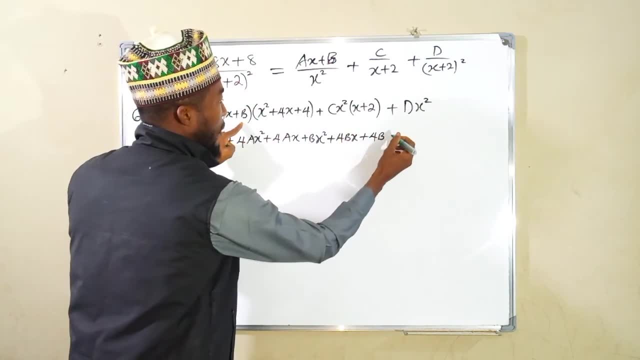 Then b times 4 is 4b. Then plus, we expand this. 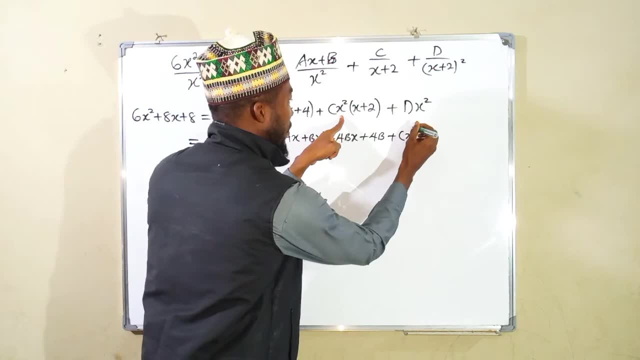 cx squared times x is going to be cx to the third power. 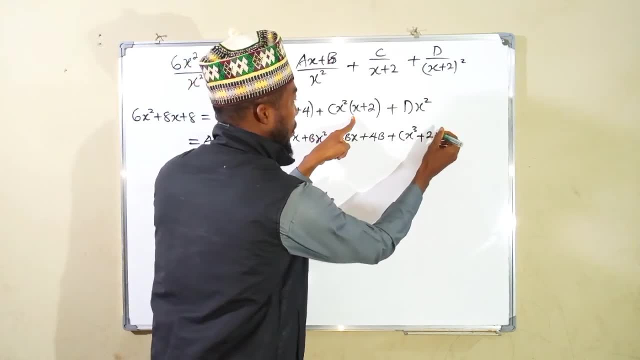 cx times 2 is going to be 2cx squared to the second power. 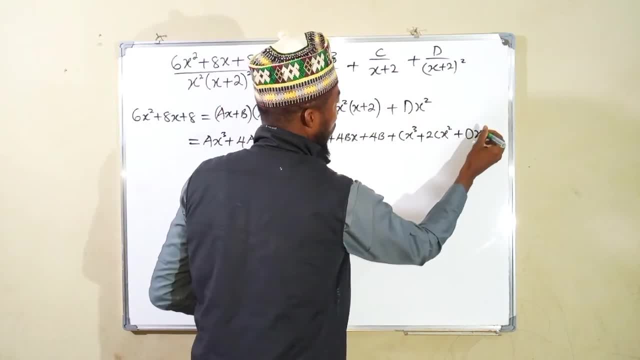 Then the last term we have dx to the second power. 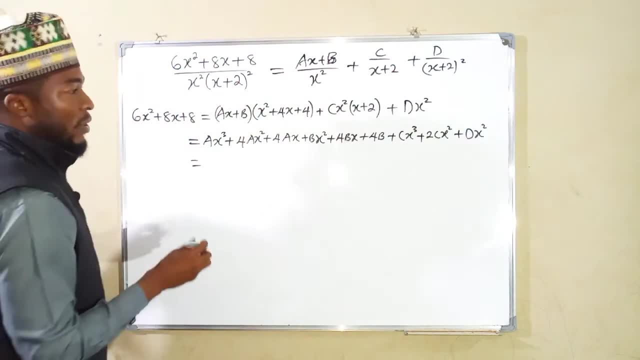 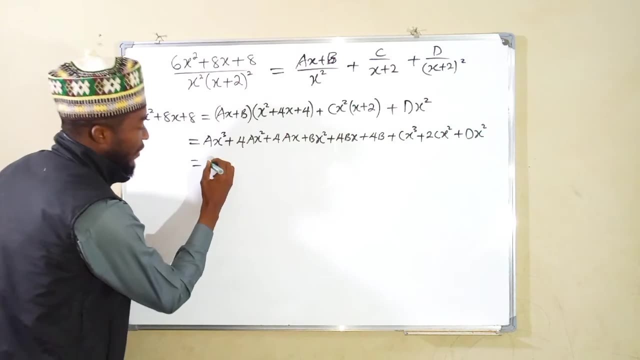 Now let us bring the like times together. Here, those with power of 3 first. We have ax to the power of 3 plus cx to the power of 3. I can factorize it by saying a plus c. 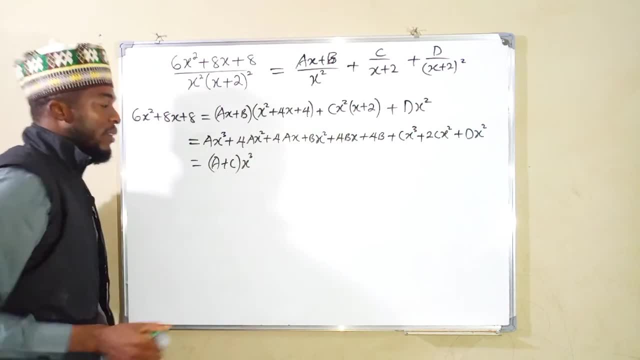 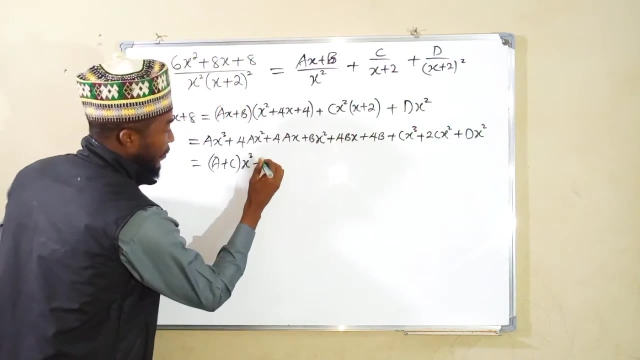 Then I will bring my x to the third power outside. Then those with power of 2, we have 1 here, 2, 3, and 4. So we can factorize it as well. Then 4a, then plus b. 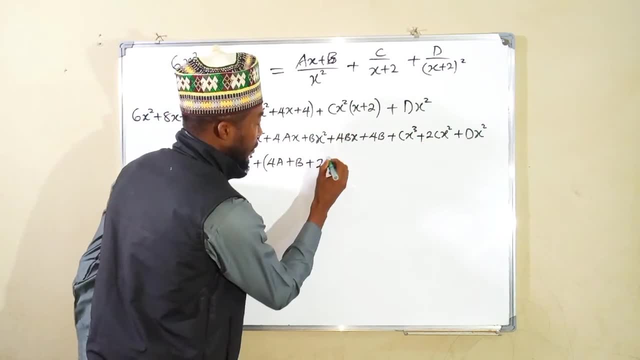 And plus. Plus 2c, then plus d. 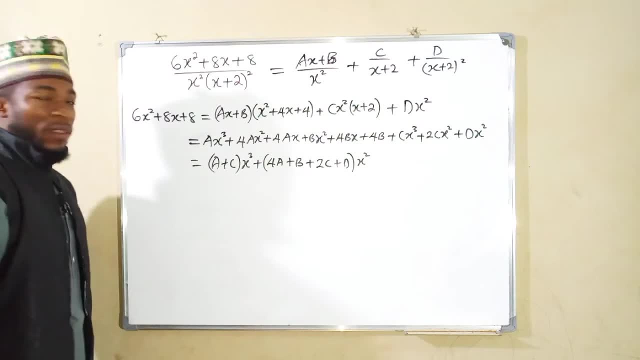 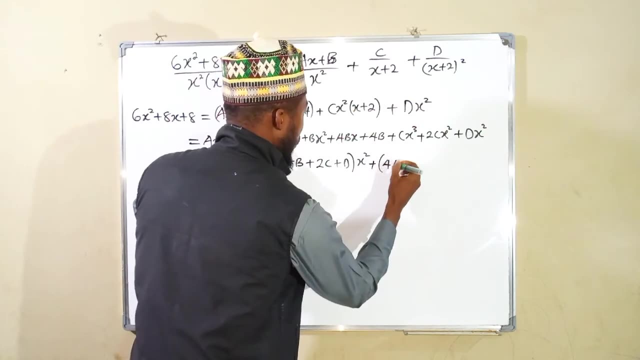 Then my x to the second power outside. Then those with x to the power of 1, we have plus 4a, 4b. My x outside. 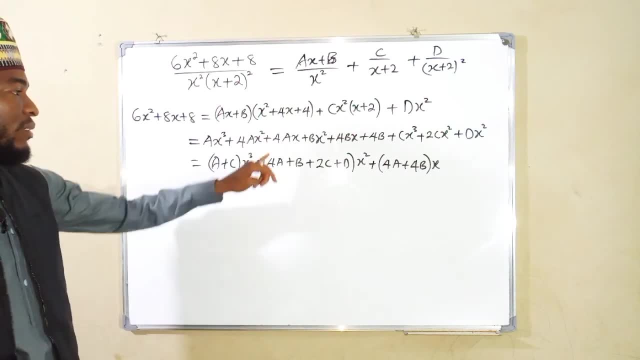 Then those. Then those without x, those constants. 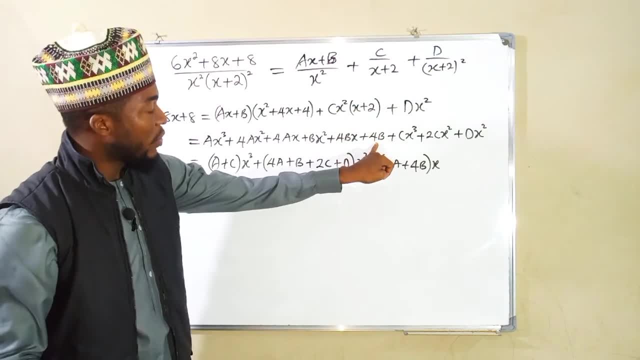 We have 4b. I think we only have 4b. 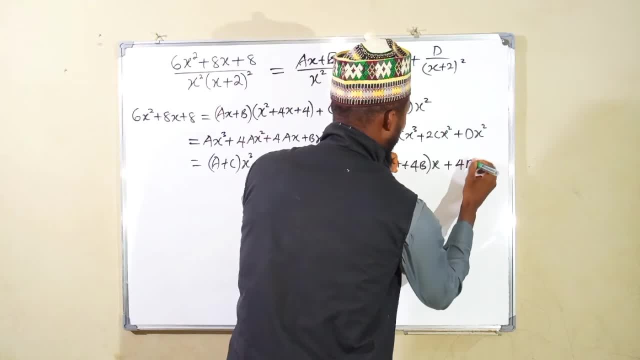 So, plus 4b. All right. 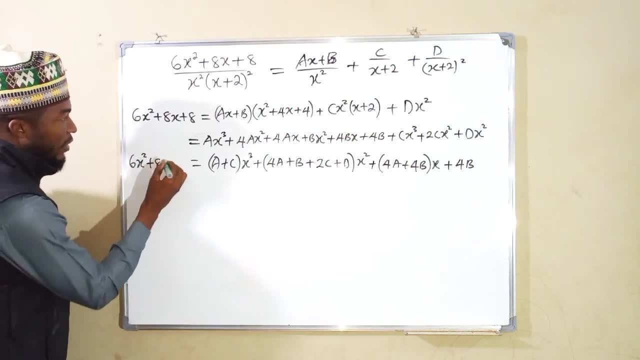 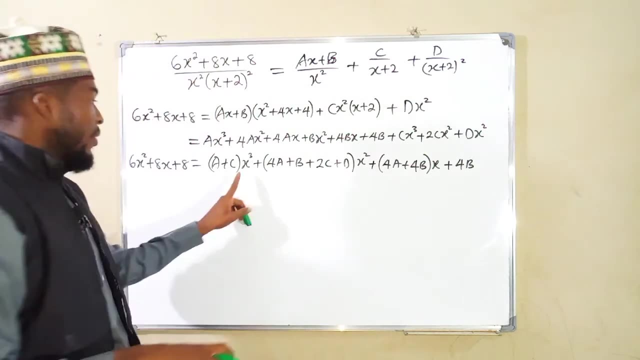 To the left, we have 6x squared plus 8x plus 8. What we are going to do, we are going to relate their coefficients. You can see we do not have x to the third power here. And hence, we are going to say, 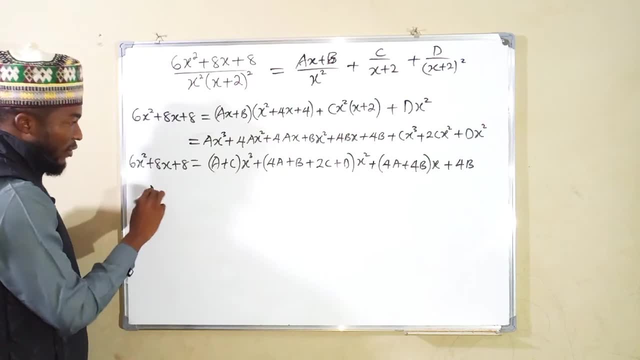 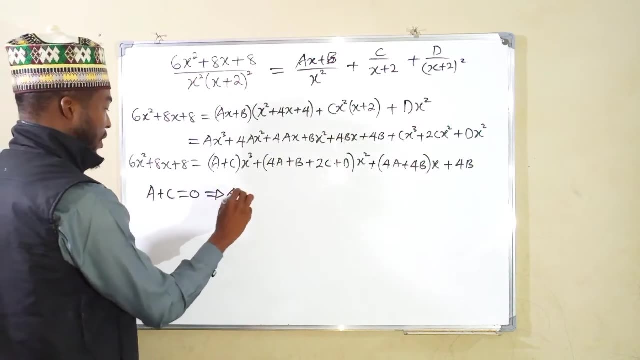 a plus c is equal to 0. Our first equation, a plus c is equal to 0, which implies that a is equal to negative c. 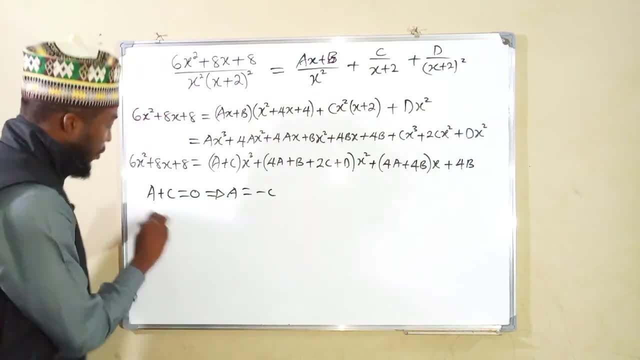 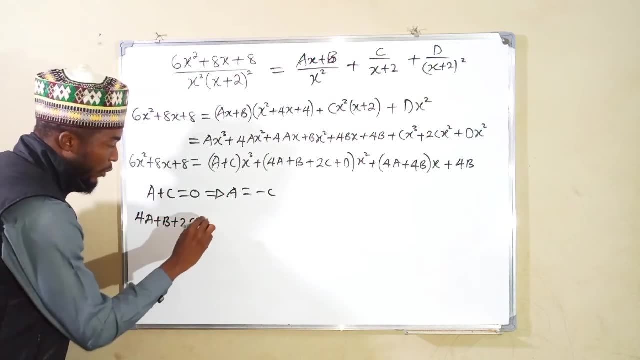 Then the coefficient of x squared to the right, we have these times, 4a plus b plus 2c plus d is going to be the coefficient of x squared to the left, which is 6. 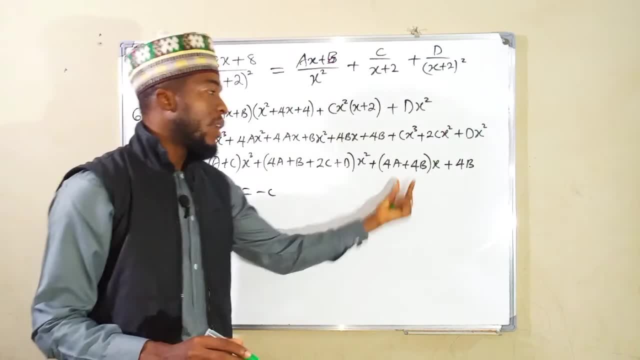 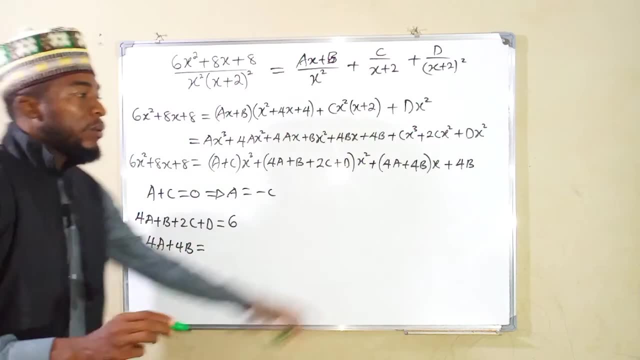 We have 4a plus 4b, 4a plus 4b, which are the coefficient of x, and we have the coefficient of x here as 8. 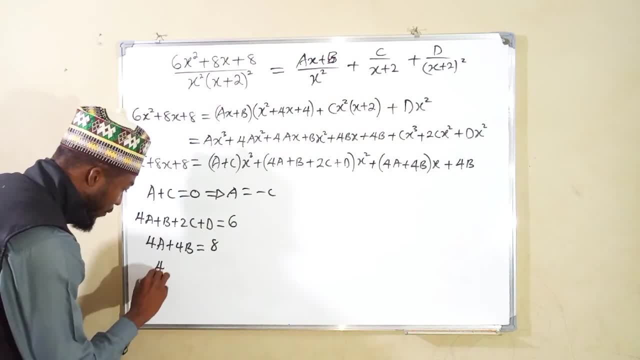 Then the constant 4b, 4b is equal to the constant to the left, 8. 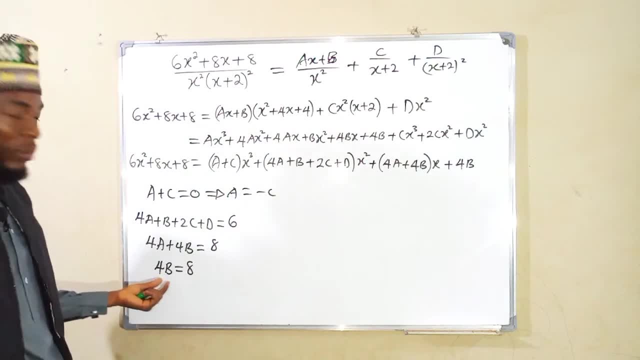 These are our equations. You can see from the last equation. 4b is equal to 8, so we can say b is equal to 2 if you divide both sides by 4. 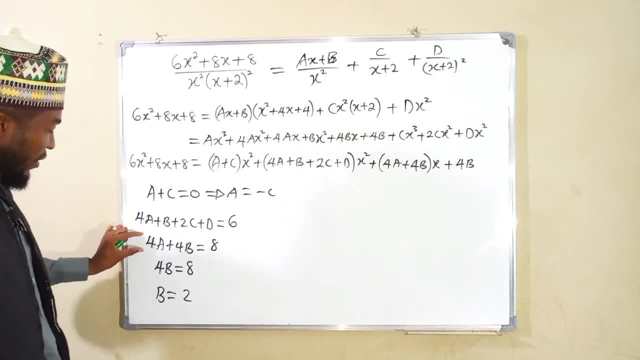 And now we can plug this b into this equation to obtain the corresponding value of a. 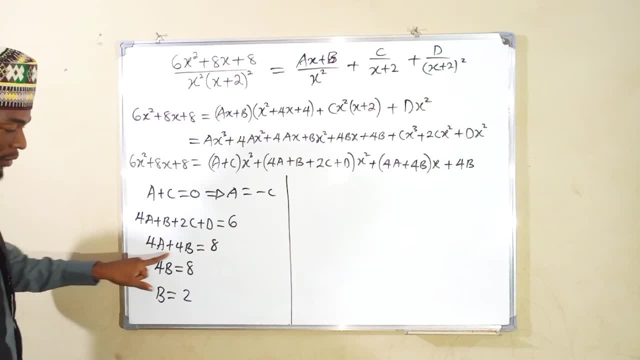 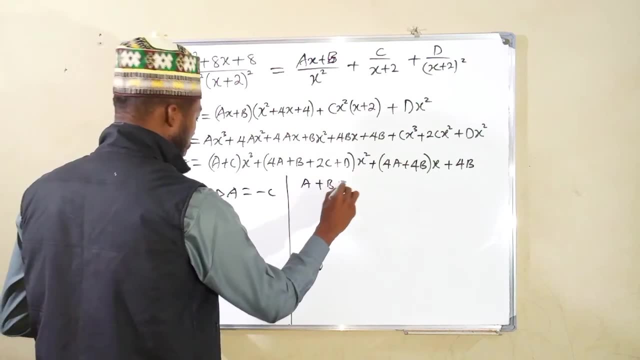 But we can equally divide each time by 4 because they have common factor. So, a plus b equals 2. If you divide. Both sides by 4. 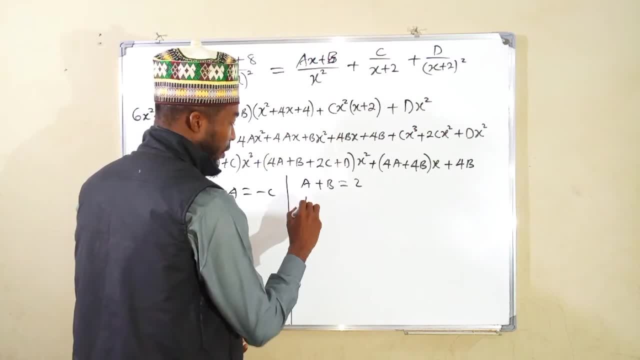 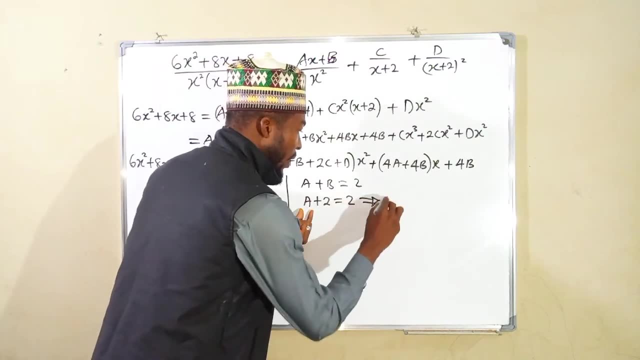 But b is equal to 2. a plus 2 equals 2. This means that a is equal to 0. 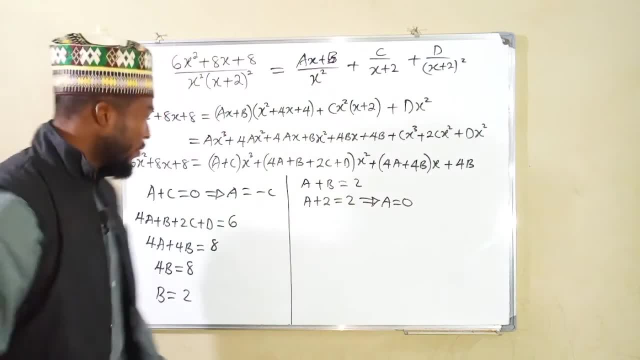 If you take 2 to the right, we say 2 minus 2, and a is equal to 0. 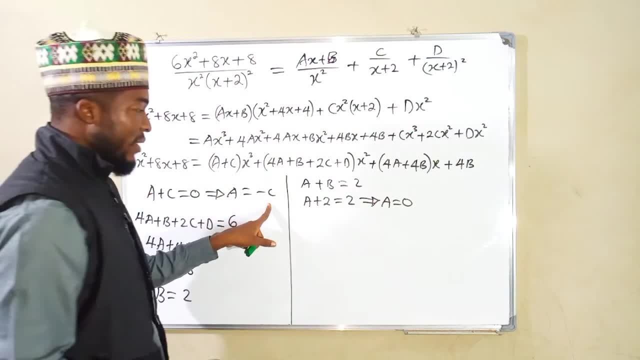 And from this equation, you can see a is equal to negative c. If a is equal to negative c. 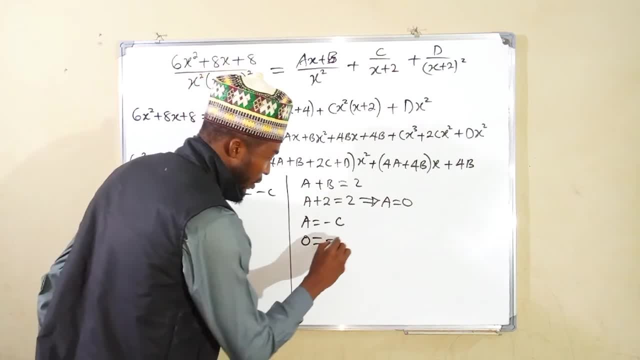 But a is 0. If you divide both sides by negative c, will also be equal to 0. 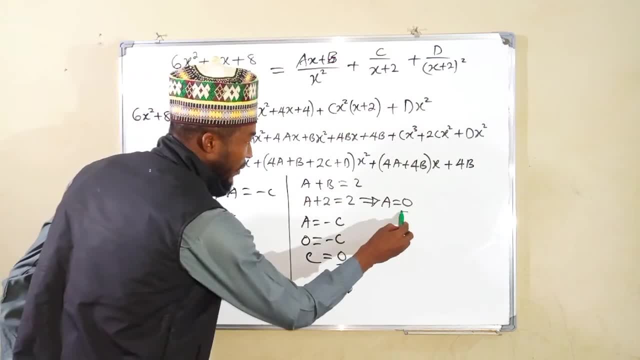 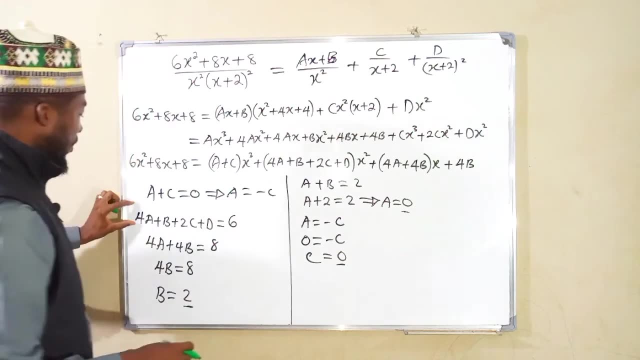 We have obtained the value of c, the value of a, the value of b. We are now going to go ahead and find the value of d. From this equation, you can see 4a. We have 4a plus b plus 2. We have 4a plus b plus 2. 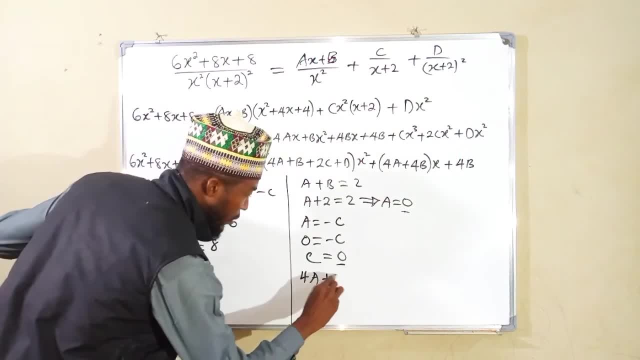 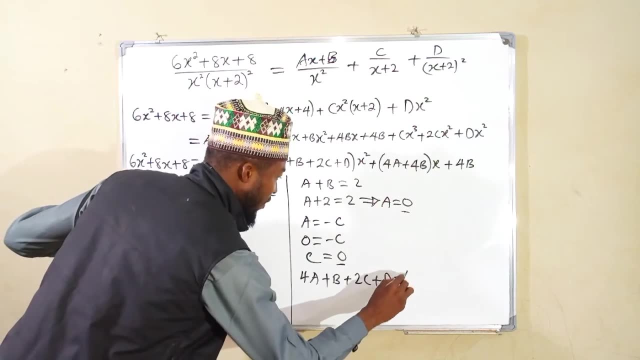 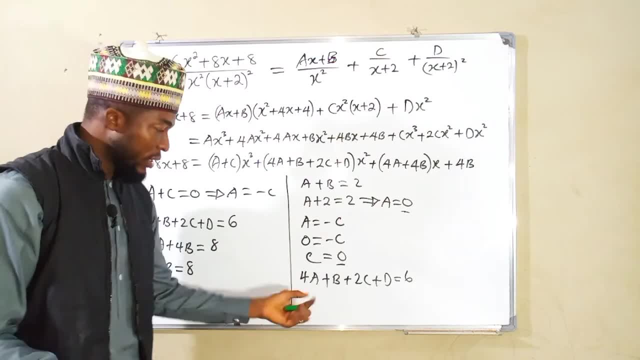 a is 0. Therefore, all this will become 0. b is 2. 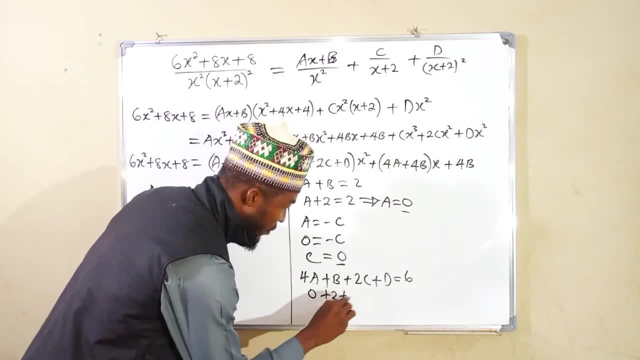 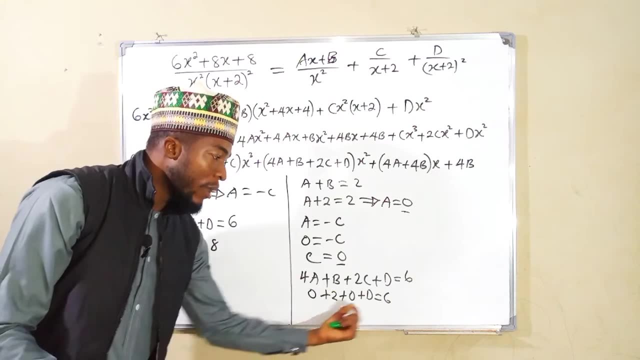 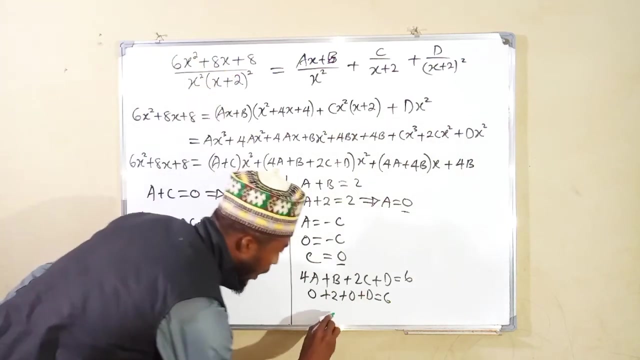 c is 0 times 2 is also 0, plus d is equal to 6. So you can see we only have 2 plus d equals 6. So to find the...? going to take 2 to the right and we say 6 minus 2 equals 4 and d now is equal to 4. 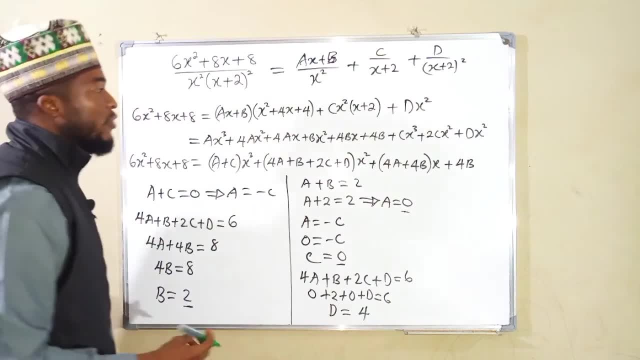 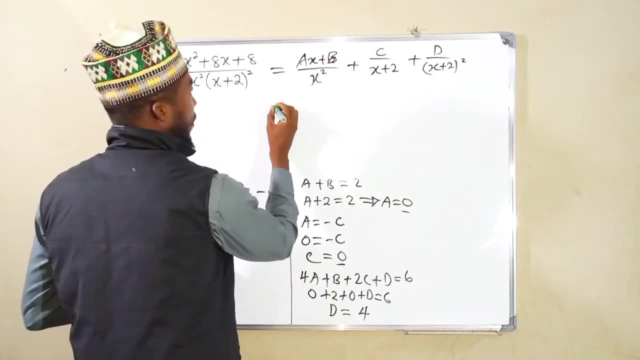 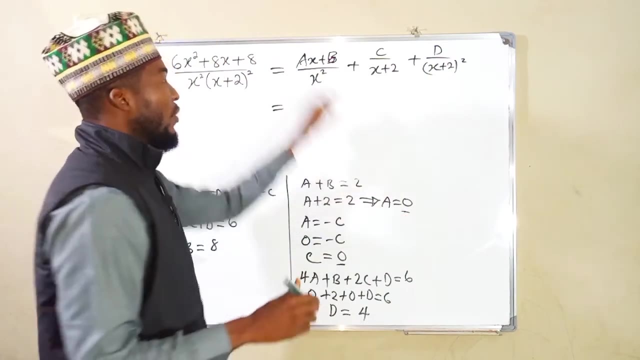 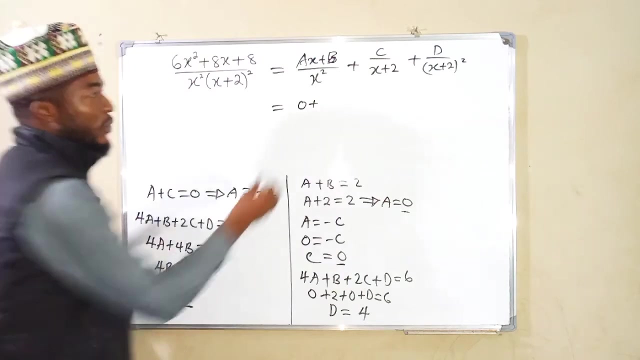 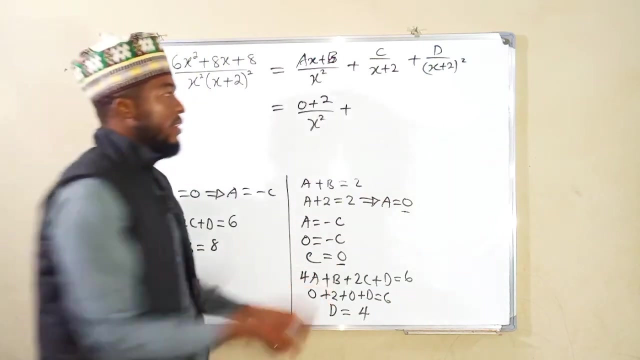 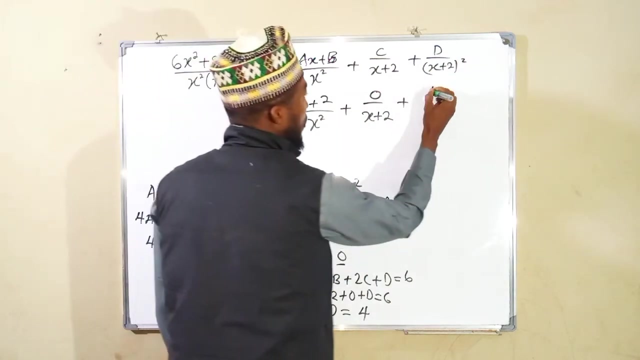 Now we have obtained all our unknown constants. Let us go back and substitute them into this expression to obtain our partial fractions. This is equal to a times x. Our a is 0 so we have 0 plus b. Our b is 2 so we have 2 over x squared plus c. You can see c is 0 over x plus 2 plus d and d is 4. The second fraction we have is 1 over x over x plus 2 to the second power. 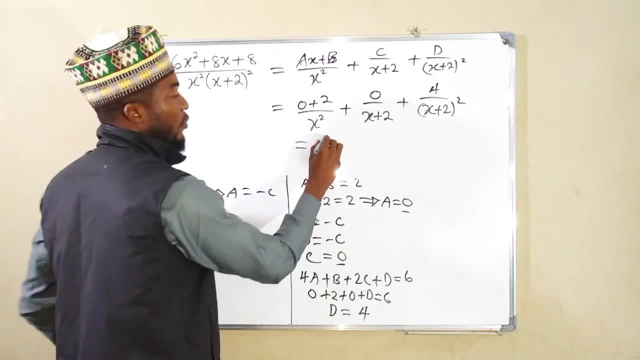 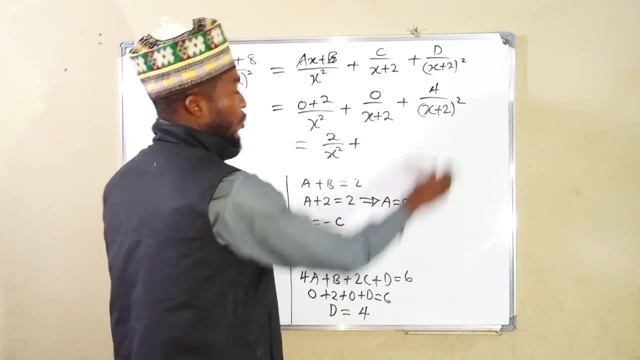 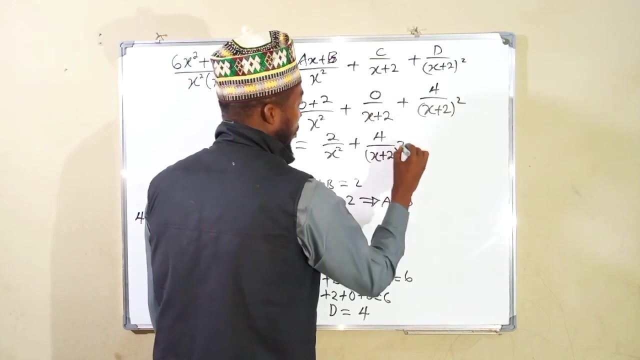 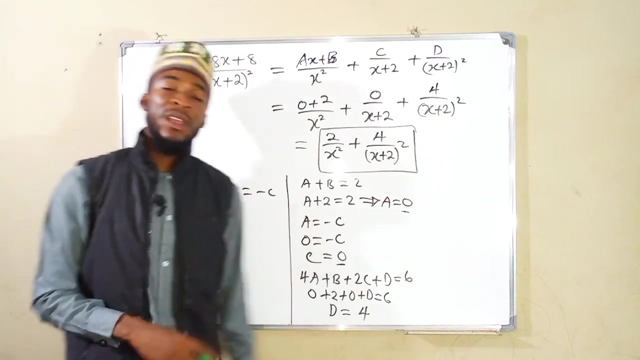 And hence we can simplify this as. 00 plus 2 is 2 over x squared plus d. The whole of this becomes 0 because the numerator is 0 and we only have the last time for 4 over x plus 2 to the second power. And hence this is our partial fraction and of this compound fraction. And this is our partial fraction. is all I have for you today thank you for watching do have a nice day